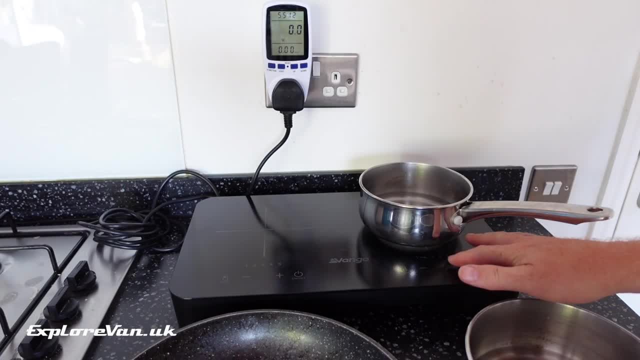 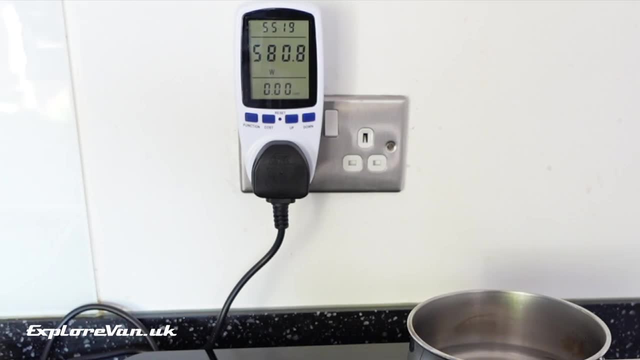 Each hob has five levels of heat and we'll talk more about those later. Here we're running on full power and you can see that with this pan it is using just under 600 watts of power. Now on the same setting, but with a larger version of the same pan. 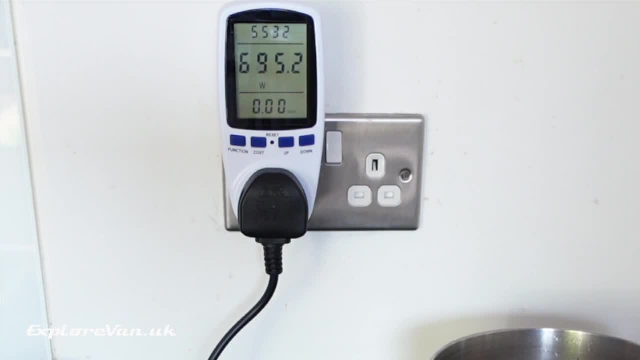 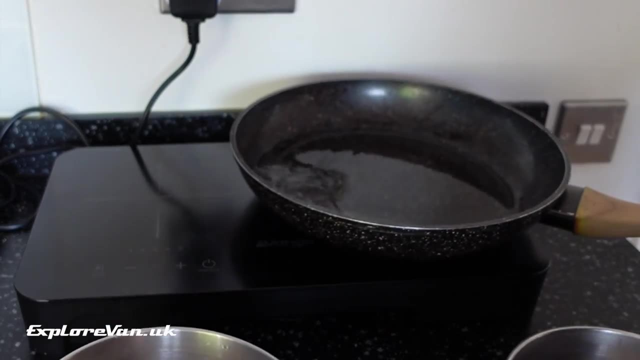 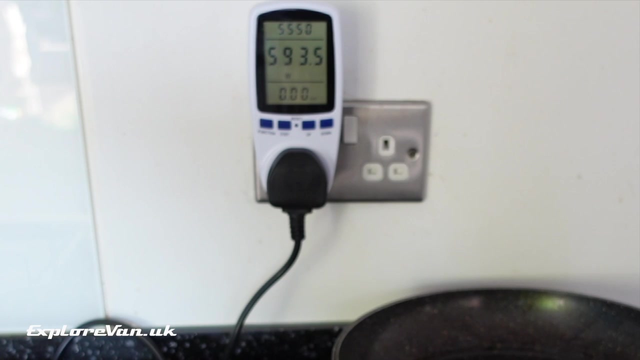 you can see that it uses more power at around 700 watts. You may think from this: the bigger the pan, the more power, but here we try a large frying pan and this actually only uses around 600 watts again. so it must be down not only to the size but the actual composition of the base. 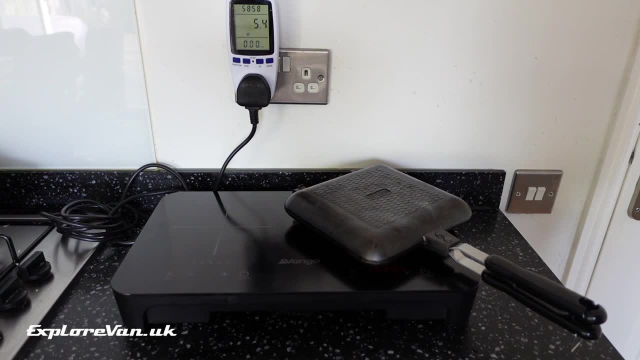 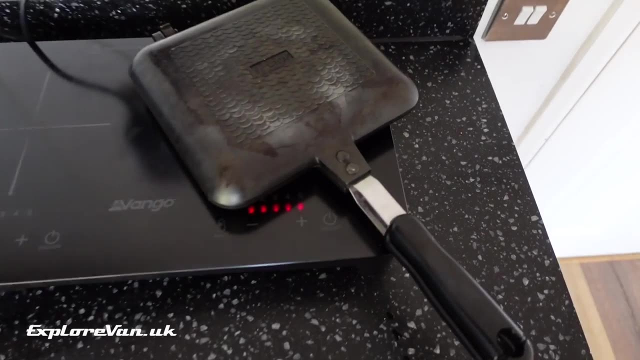 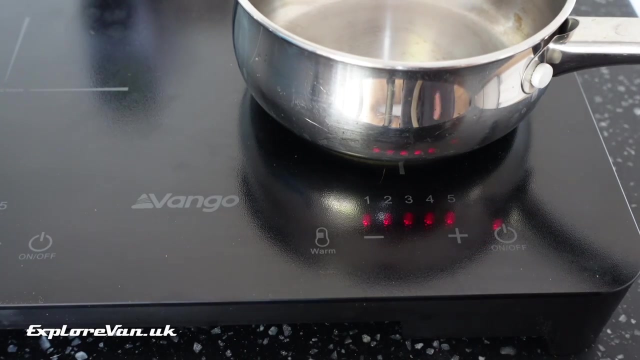 As we mentioned earlier, you must use compatible cookware. If you do try to use a non-compatible pan, the hob will beep at you, won't power up and will indicate with a flashing light After switching on the unit. setting the power is easy. 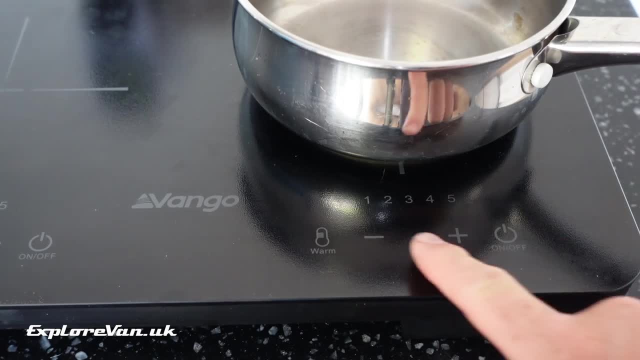 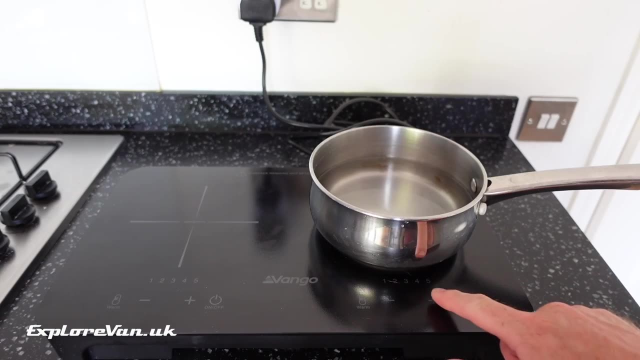 and then you can adjust it up or down using the plus or minus. You can also start it at the lowest level, not necessarily having to start it at full. It also has a warmer function, just to keep food warm. Let's go through each of the cooking levels and see how much power they use. 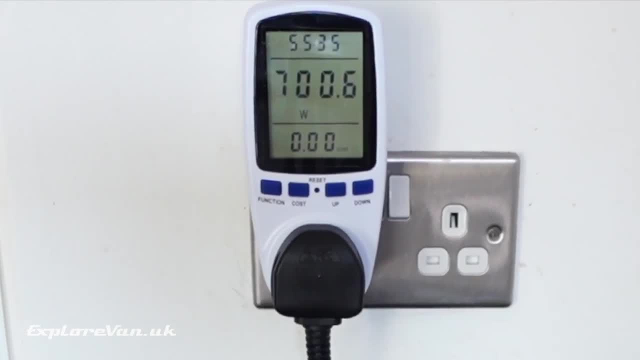 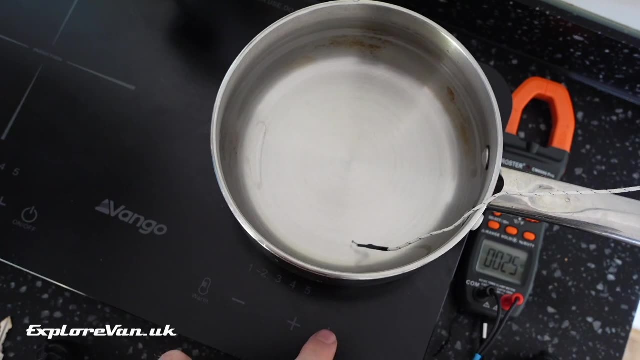 As we saw earlier, with this pan on level 5 we're just under 700 watts. Here. we've got 500 millilitres of cold water around 25 degrees out of the tap, because it's pretty warm at the moment, and let's see how long on level 5 it takes to boil. 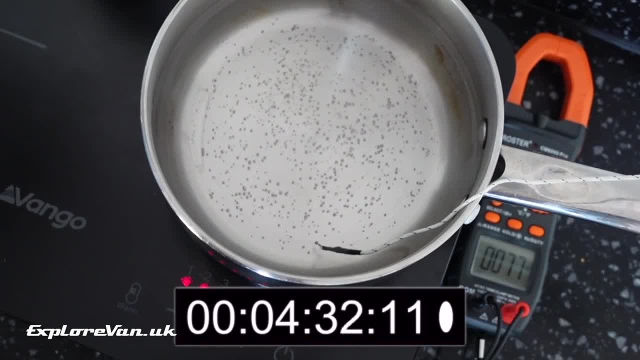 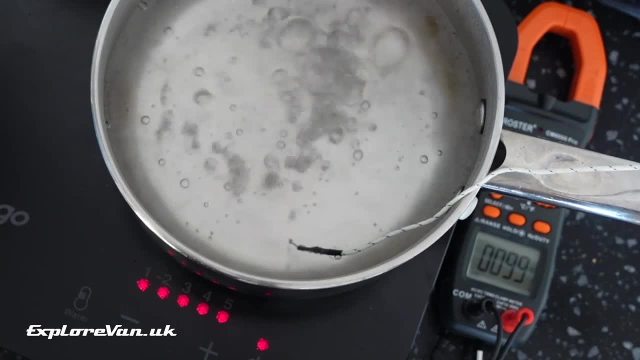 You can see I've speeded this up so it's not too boring. but you can see the temperature increasing and finally it gets to almost 100 degrees while it's boiling. If we drop the cooking level to level 4 with this pan we're just under 600 watts. 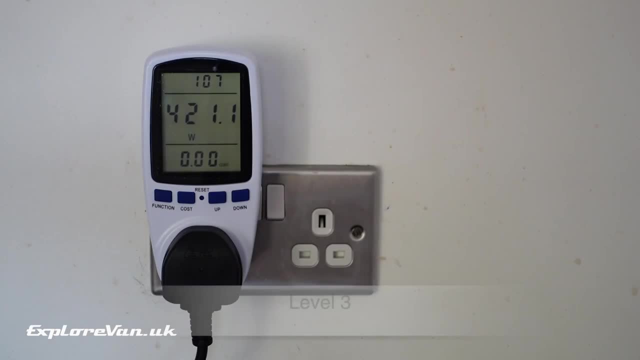 At level 3, around 400 watts. At level 2, we see a change and, rather than reducing the power to a constant level, the unit pulses the 400 watt level on and off If we drop the cooking level to level 4,. 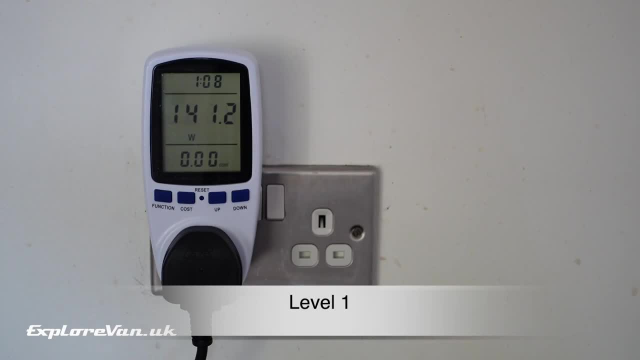 the unit pulses the 400 watt level on and off. The unit pulses the 400 watt level on and off And level 1 does similar, pulsing a 300 watt level on and off If we drop the cooking level to level 4,. 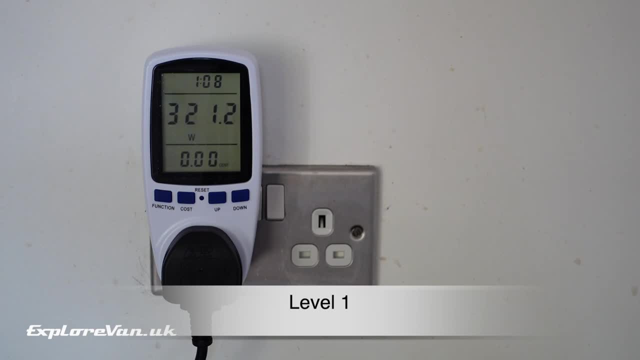 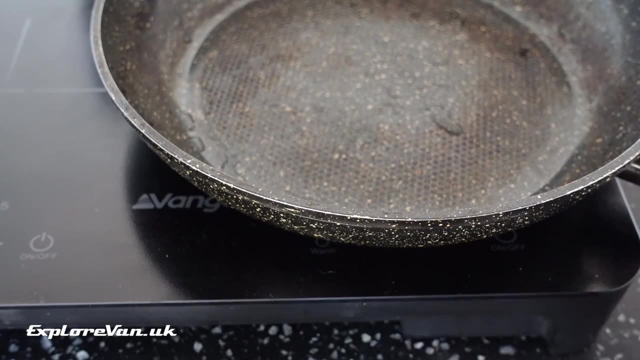 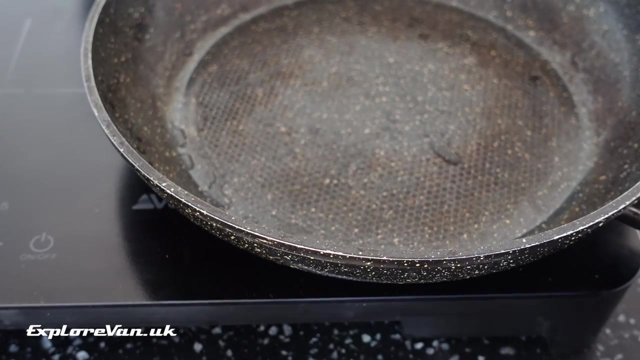 the unit pulses the 400 watt level on and off. One point of note: because of the compact size of the hob, if you are using a large frying pan you can't get to the controls. You do have to lift the pan off to change the temperature. 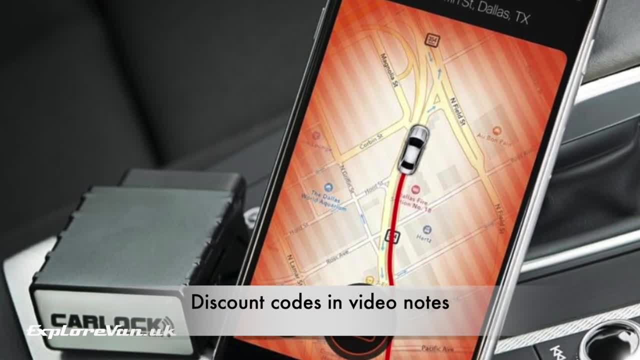 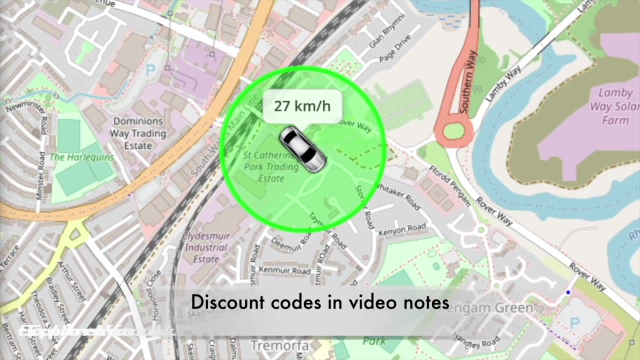 Before we look at how it performs off-grid. I'd like to say a quick thank you to Carlock for supporting this video. We've been using their advanced GPS trackers on our vehicles for some time. As they connect to multiple mobile network providers, there is a much better chance of it. 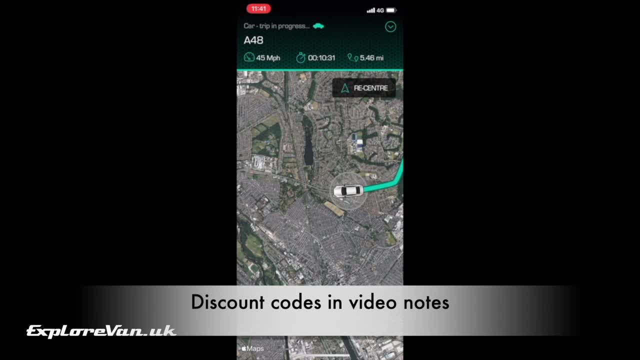 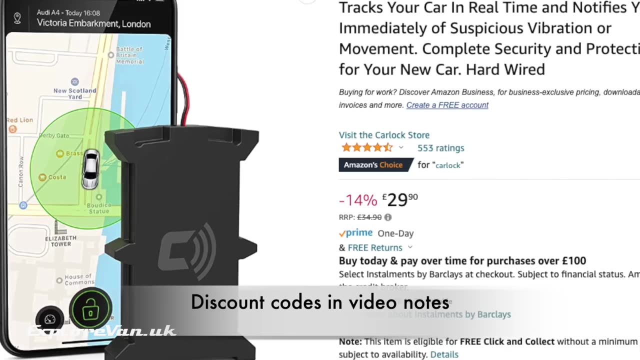 maintaining its signal, should your vehicle ever need to be tracked, Starting from only £30 for the tracker, which is simple to fit, you can get a further 10% discount by using the link and offer code in the video notes. And don't forget to also use our discount code when you activate your. 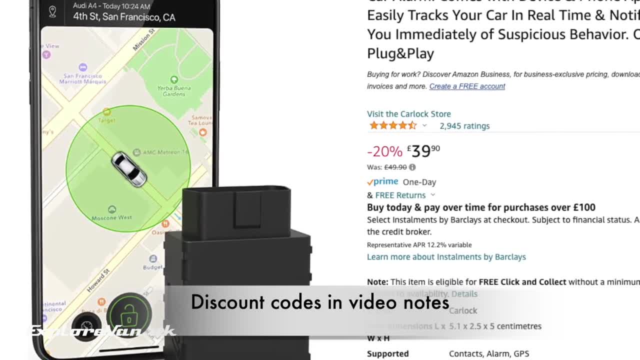 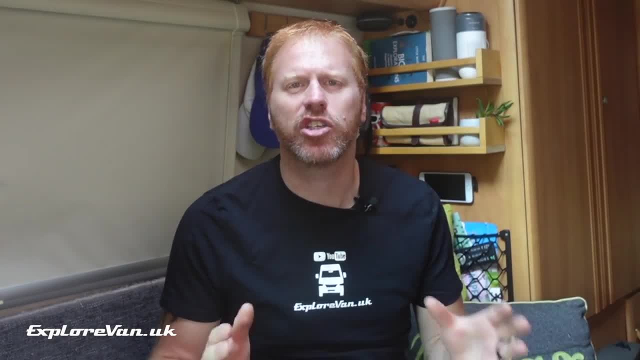 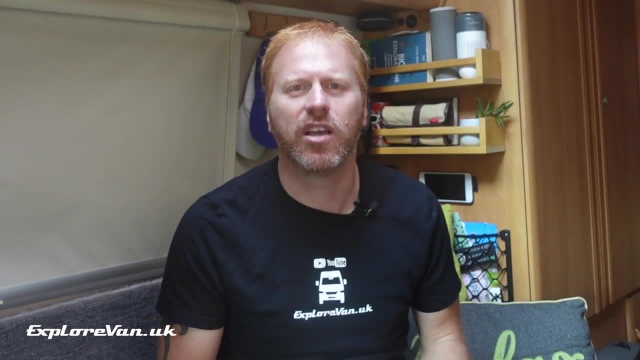 tracker, so you get extra trial subscription days for free. Now back to some off-grid cooking. We have a 200 ampere hour AGM battery bank, 280 watts of solar and a pure sine wave inverter rated at 1000 watts continuous, 2000 watts peak, Which we 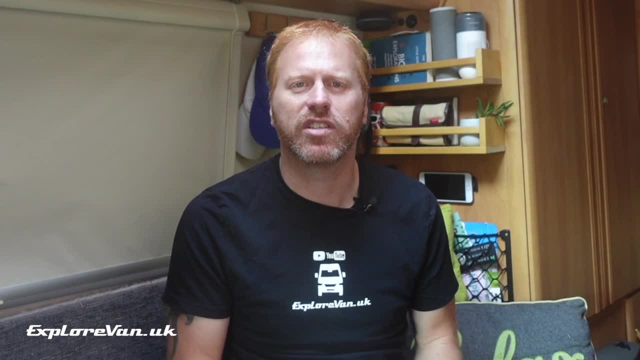 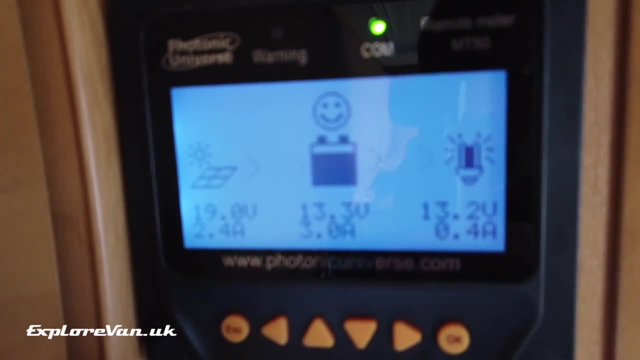 know theoretically should be capable of running one of the hobs on the sizzle. After checking, we've got a reasonably healthy battery bank and some solar power flowing. let's give it a go. We've wired our van so that we have one socket purely for hookup. 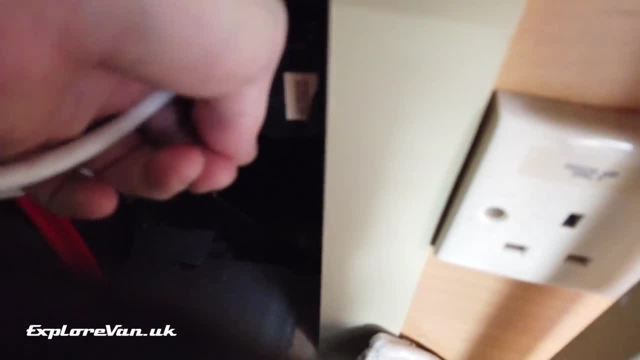 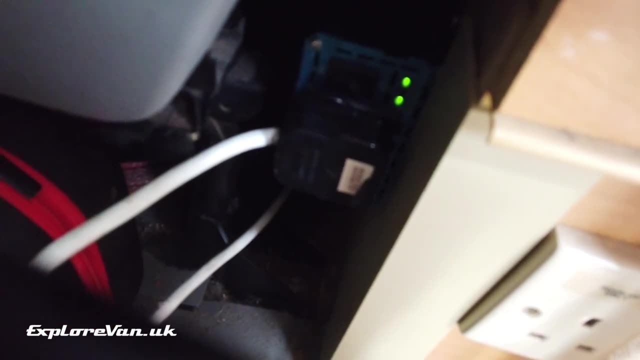 and all the other sockets run to a standard plug. That way, when we're not on hookup, by moving that plug to the inverter socket, all the other sockets in the van are powered from the inverter. We have a video on inverters coming up soon, so if this interests you, hit the subscribe. 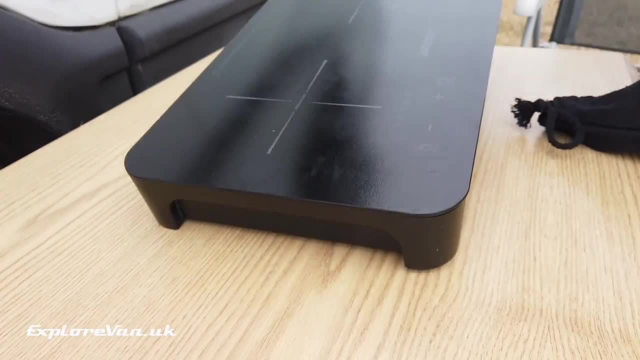 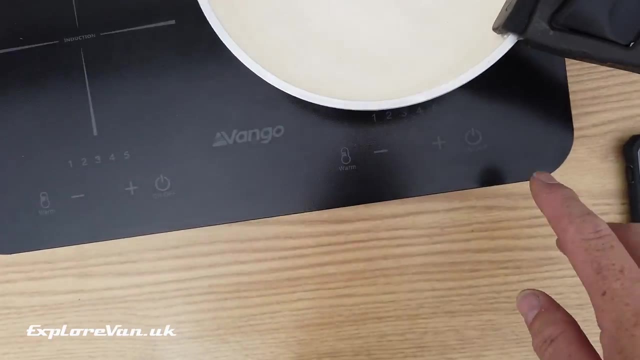 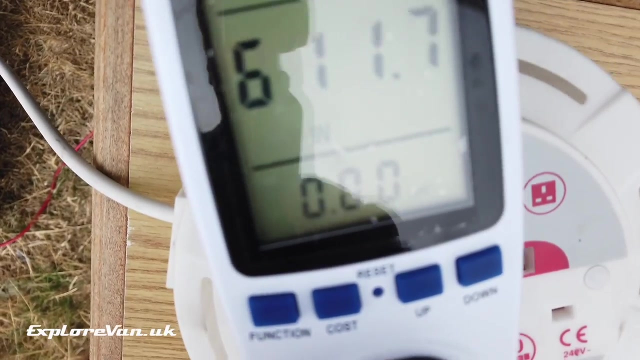 button. The hob comes with a nice cover to stop it getting damaged during transport. Our pan set from the camper van are induction compounds, so let's see how much power these use. As you can see, with this size pan we're using just over 600 watts of power. The power we are drawing has caused the battery voltage to drop, but at 12.4 volts should equate to a load of around 50 amps on the battery. But checking this, we're actually seeing 60 amps, which would suggest the inverter we're using is just over 80% efficient. 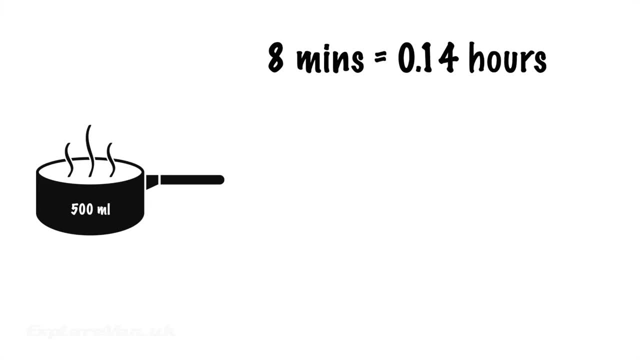 With this pan, our 500 millilitres of water took 8 minutes to boil, so that's 0.14 hours. 60 amps for 0.14 hours equates to 8.4 ampere hours, Remembering that our 200 ampere bank of AGM batteries should only be depleted to 50%.